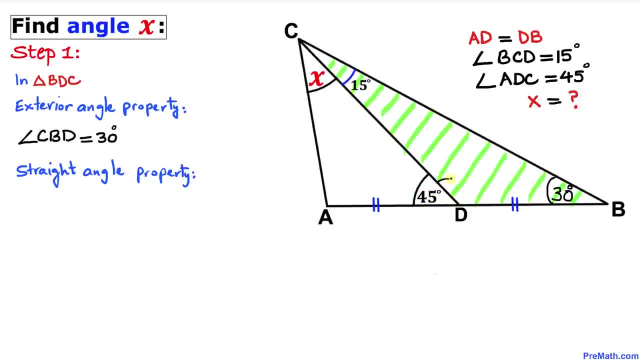 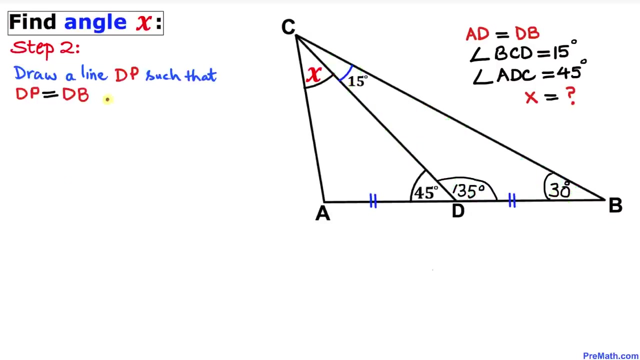 45 degrees. So therefore, this angle is going to be 135 degrees, since 135 degrees plus 45 degrees is going to make 180 degrees. Therefore, our angle BDC turns out to be 135 degrees. And here's our next step. Let's go ahead and draw a line DP such that DP. 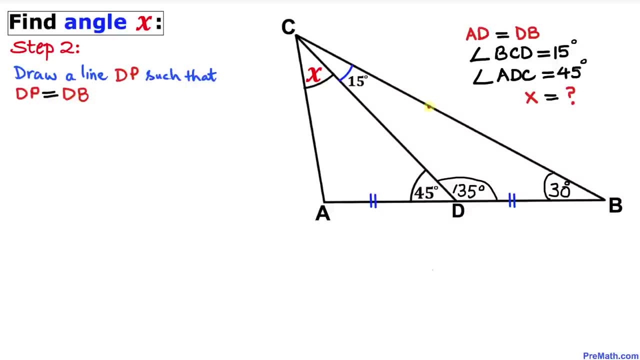 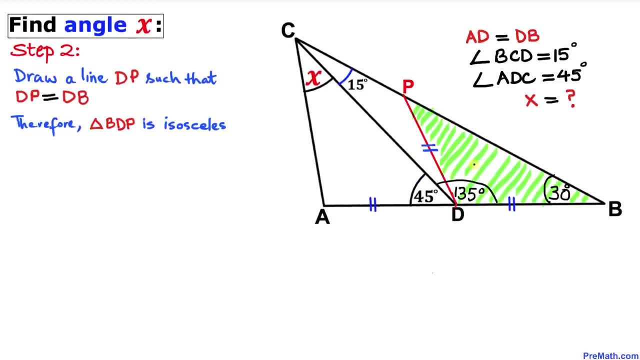 equals goes to db. let's go ahead and there's some point p is over here, such that we are going to connect this point p and d, such that this line segment and this line segment are same, and here's our much nicer looking diagram. so therefore we can see that this triangle, b, d, p is an isosceles. 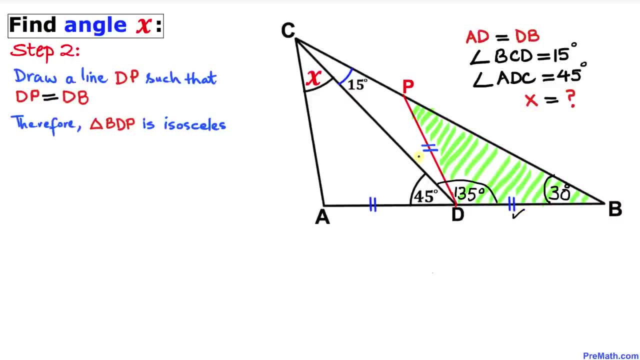 triangle, since these two sides are equal in length. so therefore, if this angle is 30 degrees, this angle has got to be 30 degrees as well. so therefore, this angle b, p, d turns out to be 30 degrees. now let's recall the angle sum property of a triangle. we know that all these three angles 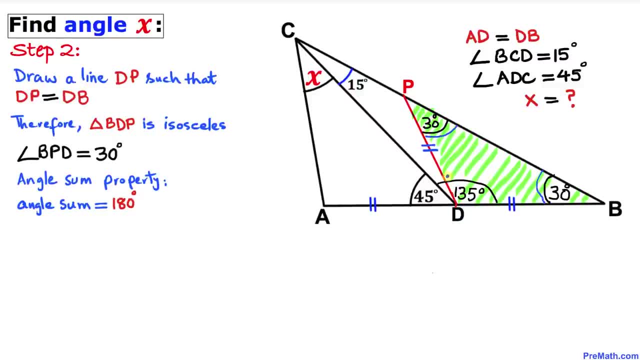 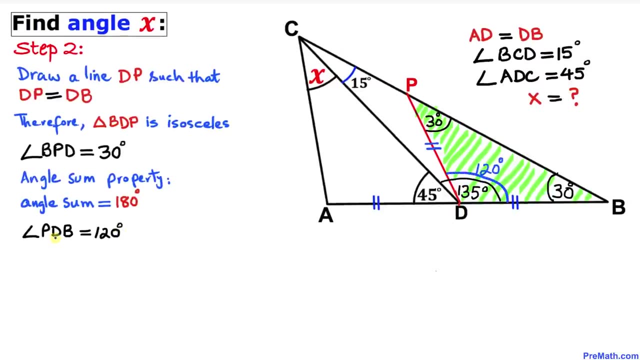 the sum of these three angles must be equal to 180 degrees. if this is 30 degrees, this is 30 degrees. this angle has got to be 120 degrees. so therefore, our angle p d b turns out to be 120 degrees. and now let's focus. 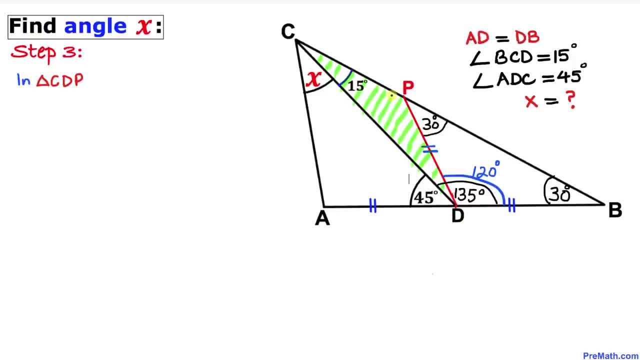 on this triangle c, d, p, and now we can see that this angle is 135 degrees and this angle is 120 degrees, so their difference, this angle, is going to be 15 degrees. so therefore, our angle c, d b turns out to be 15 degrees. now we can see that this angle is 15 degrees and this angle is 15. 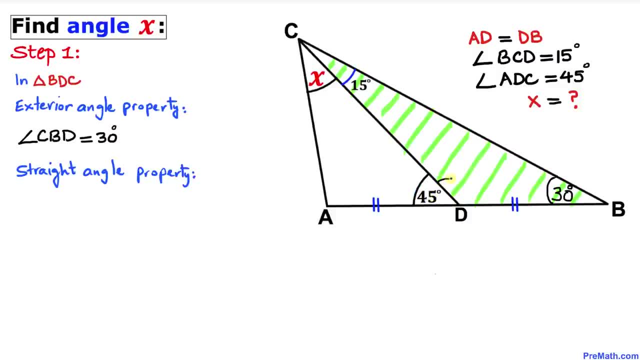 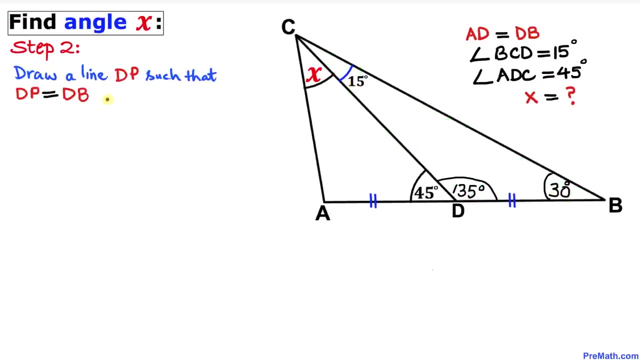 45 degrees. So therefore this angle is going to be 135 degrees, since 135 degrees plus 45 degrees is going to make 180 degrees. So therefore our angle BDC turns out to be 135 degrees. And here's our next step. Let's go ahead and draw a line DP such that DP equals DSR. 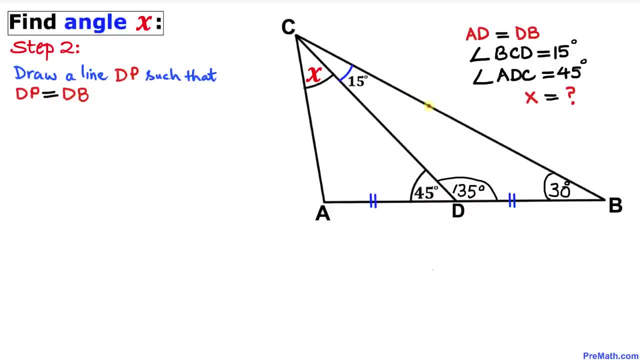 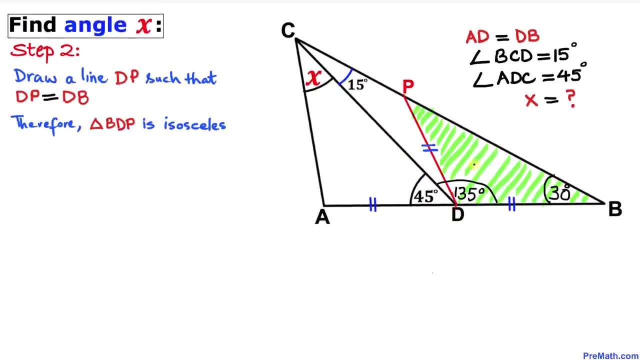 goes to db. let's go ahead, and there's some point p is over here, such that we are going to connect this point p and d such that this line segment and this line segment are same, and here's our much nicer looking diagram. so therefore we can see that this triangle b, d, p is an isosceles. 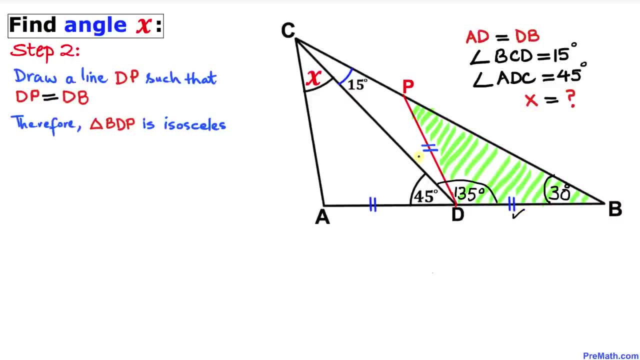 triangle, since these two sides are equal in length. so therefore, if this angle is 30 degrees, this angle has got to be 30 degrees as well. so therefore, this angle b, p, d turns out to be 30 degrees. now let's recall the angle sum property of a triangle. we know that all these three angles 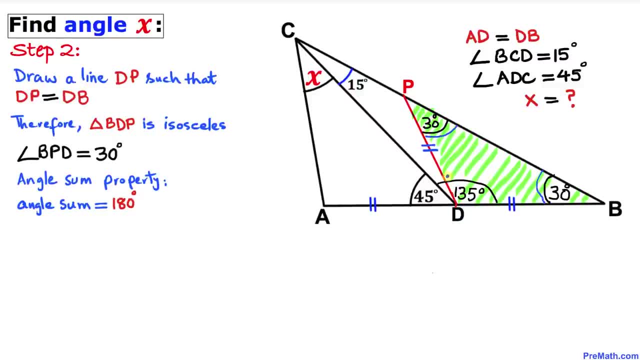 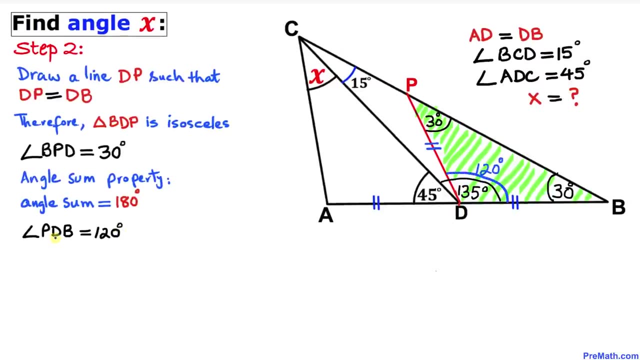 the sum of these three angles must be equal to 180 degrees. if this is 30 degrees, this is 30 degrees. this angle has got to be 120 degrees. so therefore, our angle p d b turns out to be 120 degrees. and now let's focus. 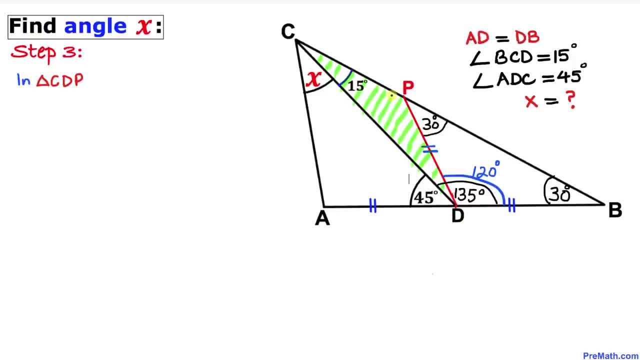 on this triangle c, d, p, and now we can see that this angle is 135 degrees and this angle is 120 degrees, so their difference, this angle, is going to be 15 degrees. so therefore, our angle c, d b turns out to be 15 degrees. now we can see that this angle is 15 degrees and this angle is 15. 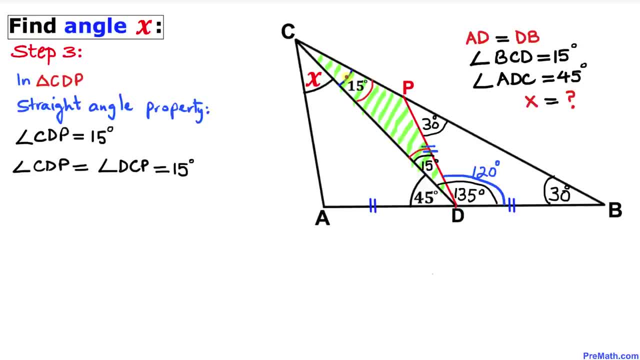 degrees as well, since these two angles are same. so that means these two sides are equal in length. this side and this side are going to be equal as well. therefore, we conclude that this line, segment c p, equals to p d, as you can see over here, and in this next step, let's go ahead and connect these. 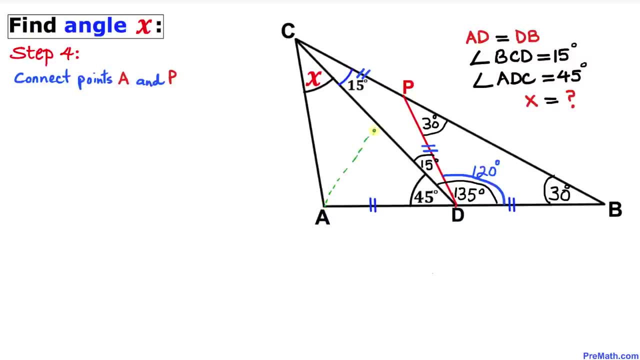 points a and p. let me just go ahead and connect these two points and here's our much nicer looking diagram. and now let's focus on this triangle a and b, and we can see that this angle is equal to a d p, and we can see that this whole angle a d p is equal to 45 degrees plus 15 degrees, that is. 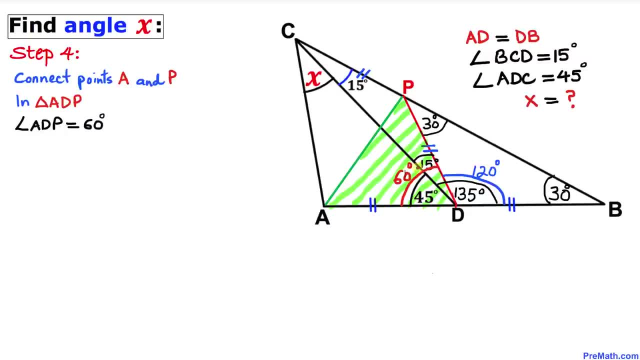 going to make it 60 degrees. now we know that this side length ad is equal to this side length dp be equal to this angle and since this angle is 60 degrees, these two angles have got to be 60 degrees each. So, therefore, this angle PAD equals to this angle APD and this angle is 60 degrees as well. 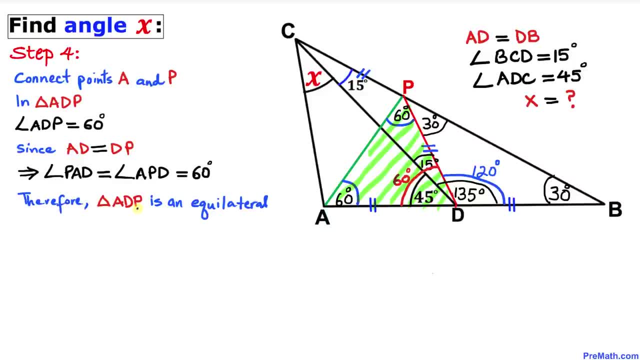 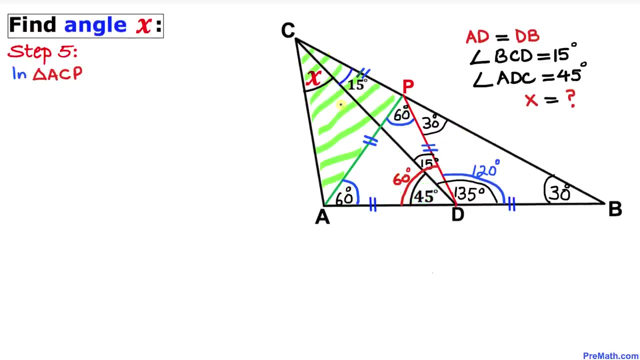 So, therefore, we conclude that this triangle, ADP is an equilateral triangle. So, therefore, this side length AP equals to this side length AD, is equal to this side length DP. And now, in this next step, let's focus on this triangle ACP. Now let's recall this: 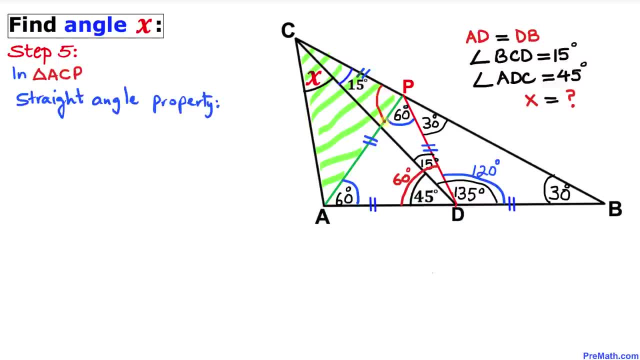 straight angle property. This whole angle is 180 degrees and since these two angles are 30 and 60 degrees, so therefore this angle has got to be 90 degrees. So therefore, our this angle APC turns out to be 90 degrees and we know that this side length C. 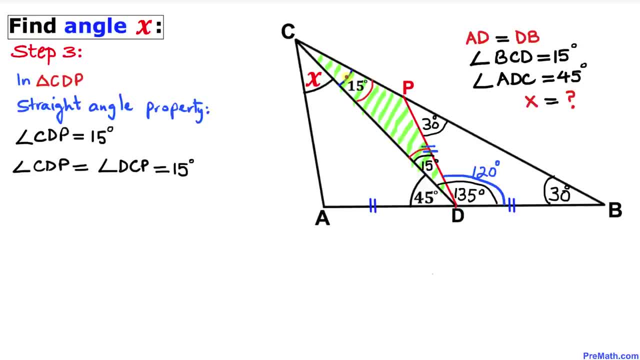 degrees as well, since these two angles are same. so that means these two sides are equal in length. this side and this side are going to be equal as well. therefore, we conclude that this line, segment c p, equals to p d, as you can see over here, and in this next step, let's go ahead and connect these. 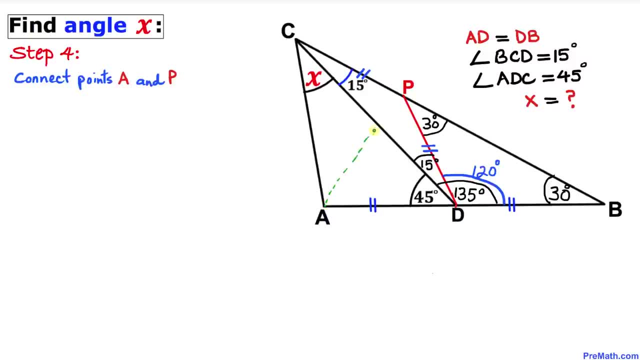 points a and p. let me just go ahead and connect these two points and here's our much nicer looking diagram. and now let's focus on this triangle a and b, and we can see that this angle is equal to a d p, and we can see that this whole angle a d p is equal to 45 degrees plus 15 degrees, that is. 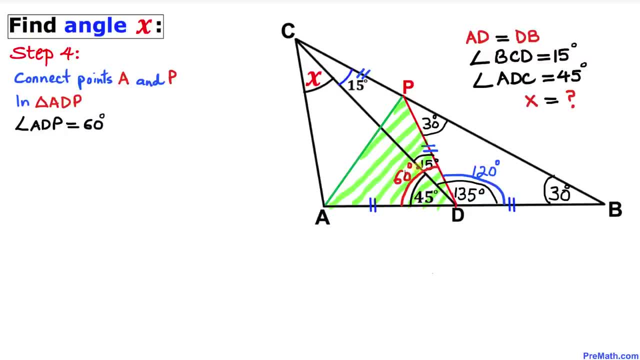 going to make it 60 degrees. now we know that this side length a, d is equal to this side length d, p. so therefore, this angle is going to make this angle 60 degrees, or the angle had to be 60 degrees, be equal to this angle and since this angle is 60 degrees, these two angles have got to be 60 degrees. 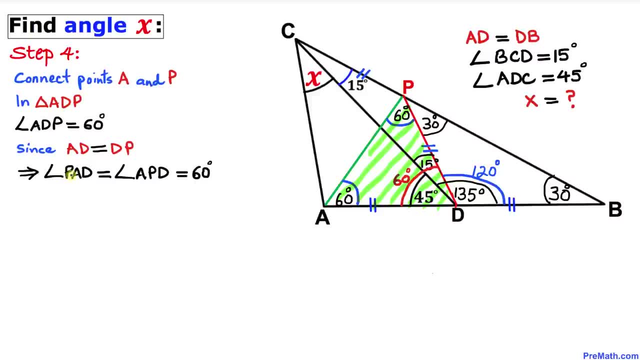 each. So therefore this angle PAD, equals to this angle APD, and this angle is 60 degrees as well, So therefore we conclude that this triangle, ADP, is an equilateral triangle, So therefore this side length AP equals to this side length, AD is equal to this side length. 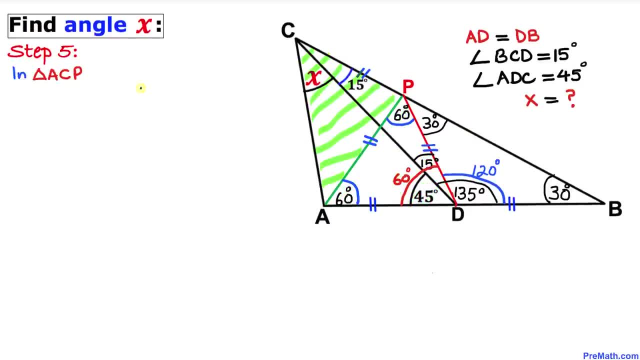 DP. And now, in this next step, let's focus on this triangle ACP. Now let's recall this straight angle property. This whole angle is 180 degrees and since these two angles are 30 and 60 degrees, so therefore this angle has got to be 90 degrees. So therefore, our this angle APC turns out to be 90 degrees. 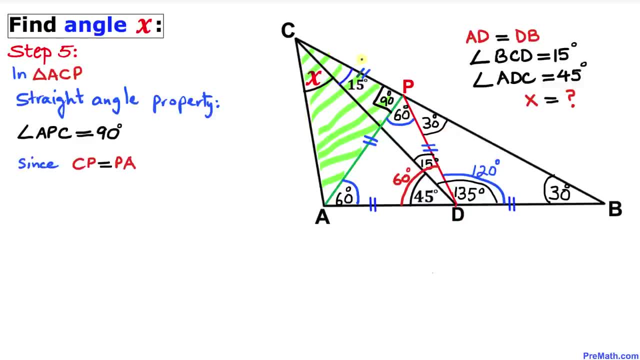 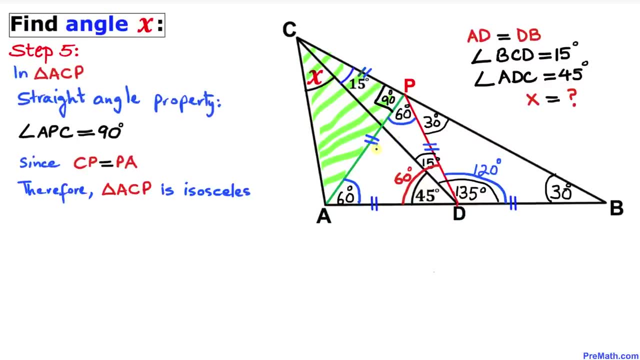 and we know that this side length C letters of angle rapid baby problem, an equilateral triangle consumption. So therefore this angle APC turns out to be 90 degrees and we know that this side length C is equal to this side length PA. therefore we conclude that this triangle ACP is an isosceles. 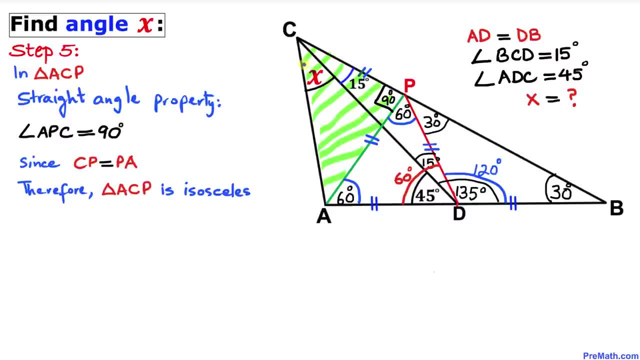 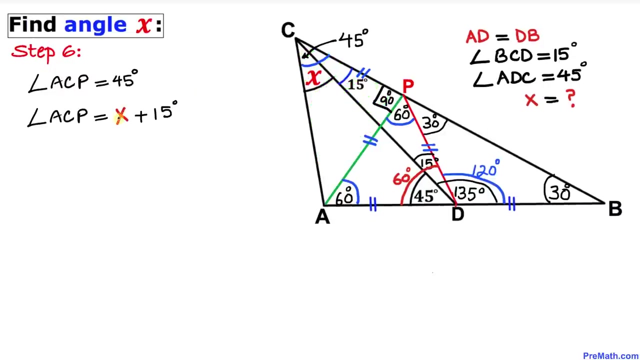 triangle. so, therefore, we conclude that this angle and this angle, they are equal. and since this angle is 90 degrees, these both angles are going to be 45 degree and this angle is going to be 45 degrees as well. so, therefore, our this angle ACP turns out to be 45 degrees. and here's our final step. 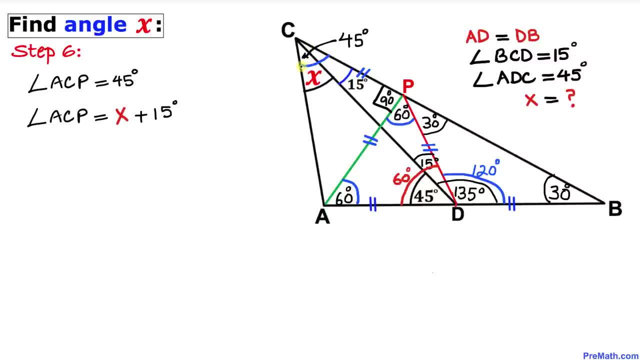 our angle ACP. this angle is 45 degrees, as we can see, and this angle ACP turns out to be 45 degrees, as we can see, and this angle ACP turns out to be 45 degrees, as we can see, And this angle ACP is also equal to the sum of these two angles, X and 15 degrees. 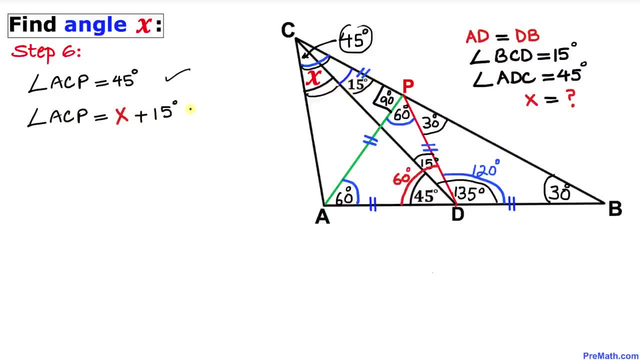 I wrote down angle: ACP equals to X plus 15 degrees, So therefore I can write this one as X plus 15 degrees equals to 45 degrees. Let's go ahead and subtract 15 degrees from both sides, So therefore these two are gone. 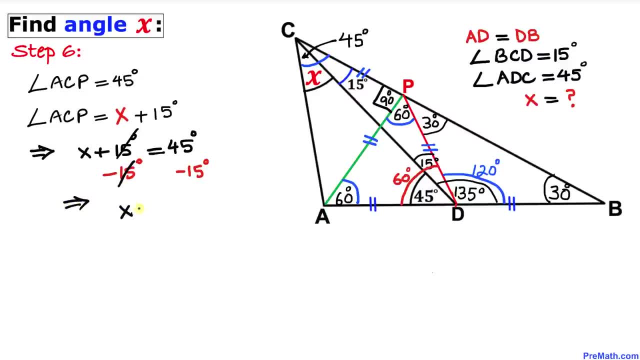 So our X value turns out to be simply 30 degrees. So that's our angle. X turns out to be 30 degrees And that's our final answer. Thanks for watching and please don't forget to subscribe to my channel for more exciting videos. 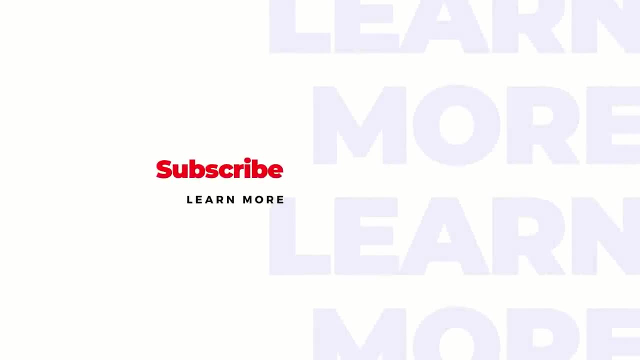 Bye. Thanks for watching.